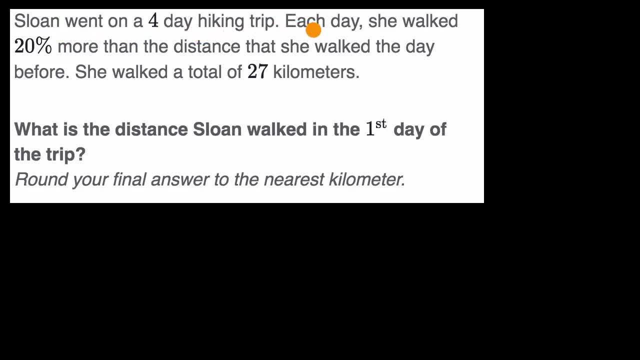 We're told, Sloan went on a four-day hiking trip. Each day she walked 20% more than the distance that she walked the day before. She walked a total of 27 kilometers. What is the distance Sloan walked in the first day of the trip? 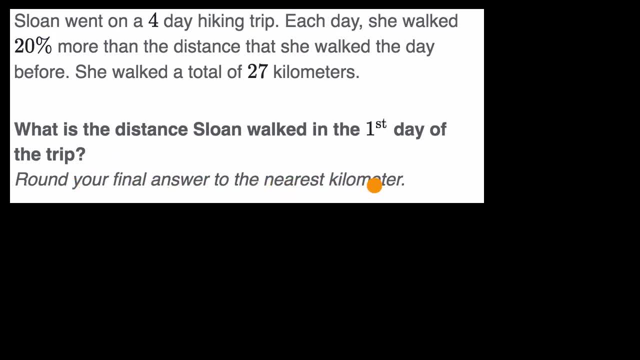 And it says: to round our final answer to the nearest kilometer. So, like always, have a go at this and see if you can figure out how much she walked on the first day. All right, well, let's just call the amount. 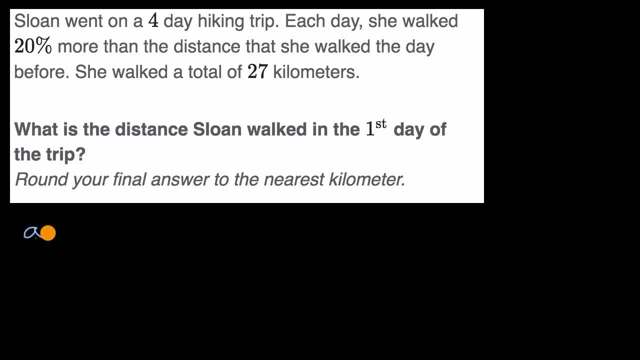 that she walked on the first day, a, And then, using a, let's see if we can set up an expression for how much she walked in total, And then that should be equal to 27, and then hopefully we're going to be able to solve for a. 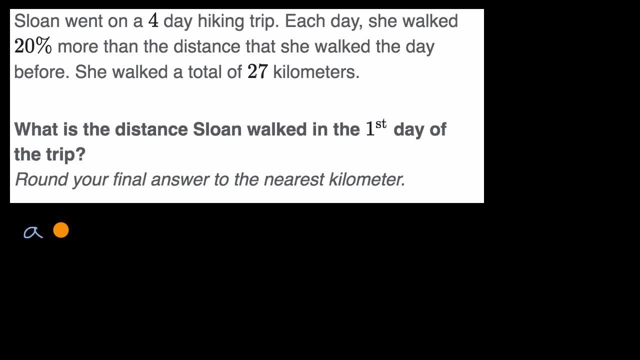 So on the first day she walks a kilometers. Now how about the second day? Well, they tell us that each day she walked 20% more than the distance she walked the day before. So on the next day she's going to walk. 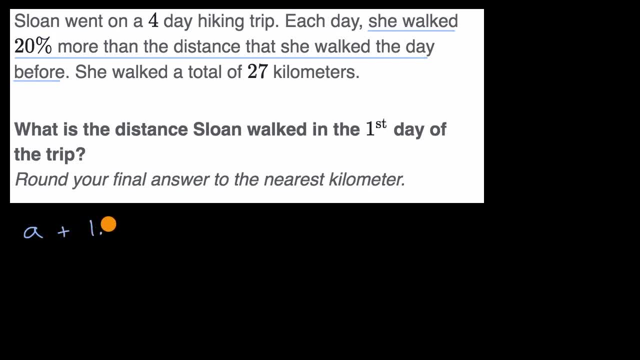 20% more than a kilometers, So that's 1.2 times a. And what about the day after that, her third day? Well, that's just going to be 1.2 times this, the second day, And so that's going to be 1.2 times 1.2,. 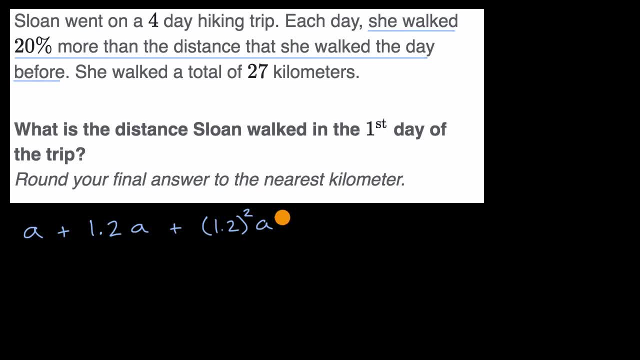 or we could say 1.2 squared times a. And then how much on the fourth day, And that's she went on a four-day hiking trip. so that's the last day. Well, that's going to be 1.2 times the third day. 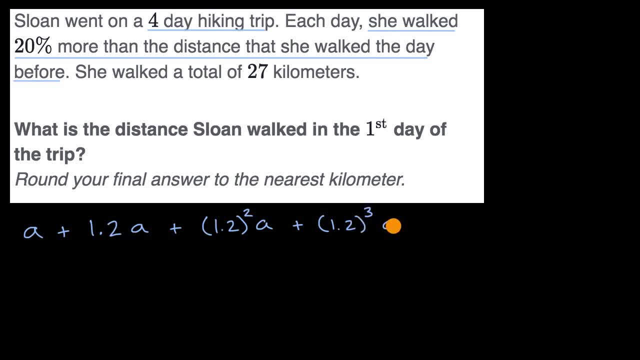 So that's going to be 1.2 to the third power times, a. So this is an expression in a on how much she walked over the four days, And we know that she walked a total of 27 kilometers, So this is going to be equal to 27 kilometers. 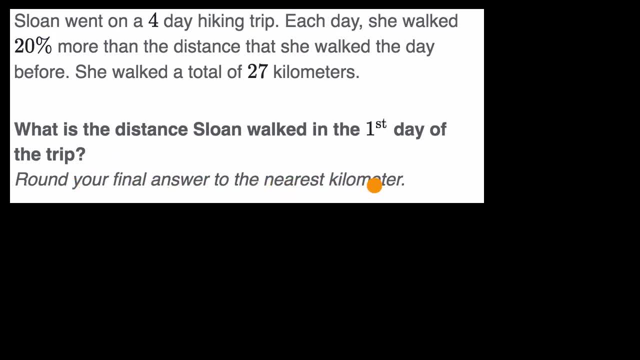 And it says: to round our final answer to the nearest kilometer. So, like always, have a go at this and see if you can figure out how much she walked on the first day. All right, well, let's just call the amount. 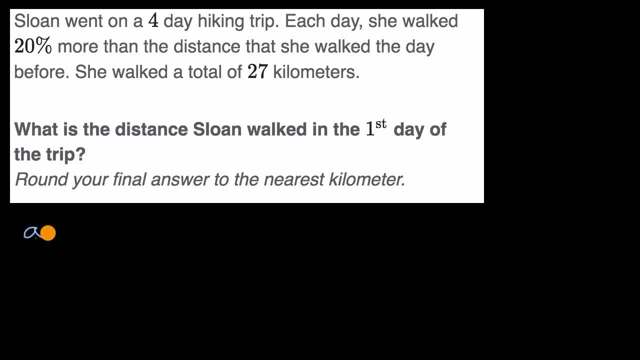 that she walked on the first day, a, And then, using a, let's see if we can set up an expression for how much she walked in total, And then that should be equal to 27, and then hopefully we're going to be able to solve for a. 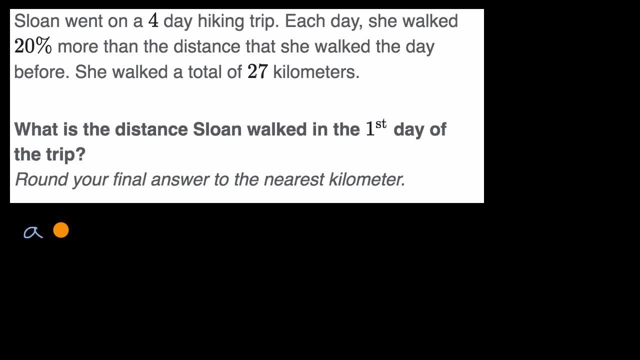 So on the first day she walks a kilometers. Now how about the second day? Well, they tell us that each day she walked 20% more than the distance she walked the day before. So on the next day she's going to walk. 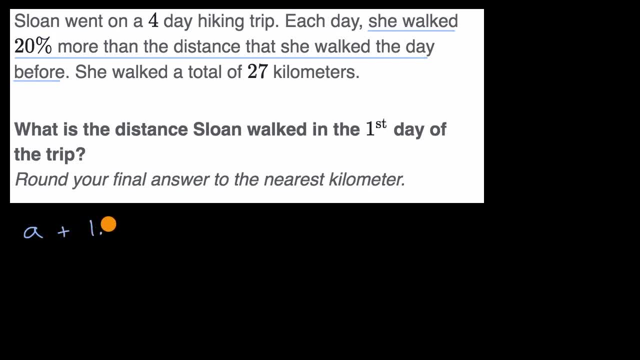 20% more than a kilometers, So that's 1.2 times a. And what about the day after that, her third day? Well, that's just going to be 1.2 times this, the second day, And so that's going to be 1.2 times 1.2,. 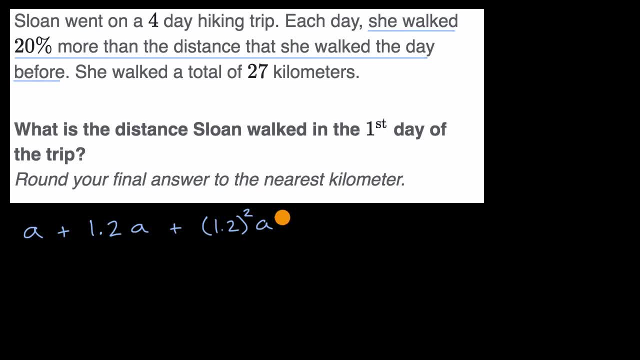 or we could say 1.2 squared times a. And then how much on the fourth day, And that's she went on a four-day hiking trip. so that's the last day. Well, that's going to be 1.2 times the third day. 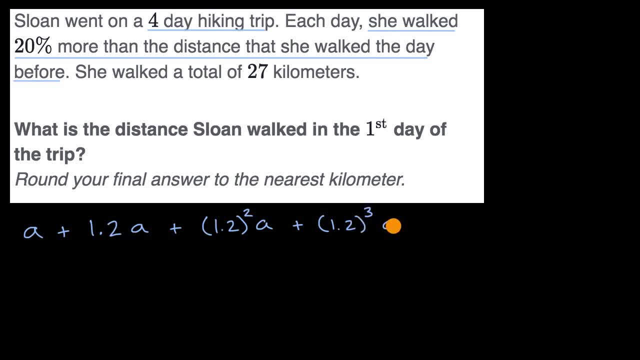 So that's going to be 1.2 to the third power times, a. So this is an expression in a on how much she walked over the four days, And we know that she walked a total of 27 kilometers, So this is going to be equal to 27 kilometers. 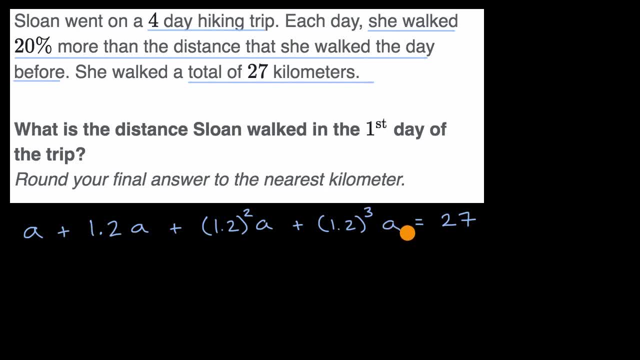 Now you could solve for a over here. You could factor out the a and you could say: a times one plus 1.2, plus 1.2 squared plus 1.2 to the third power is equal to 27.. And then you could say that a is equal to 1.2 squared. 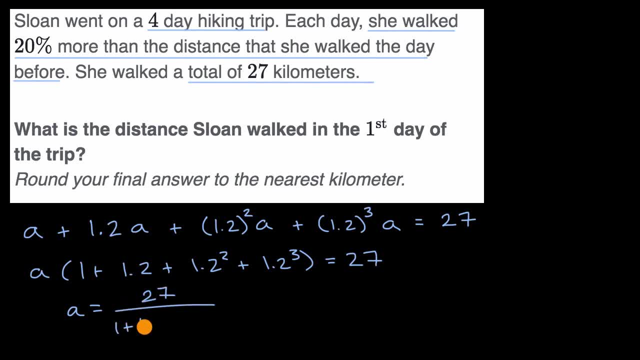 That's equal to 27 over one plus 1.2, plus 1.2 squared plus 1.2 to the third power, And we would need a calculator to evaluate this. But I'm going to do a different technique, a technique that would work even if you had 20 terms here. 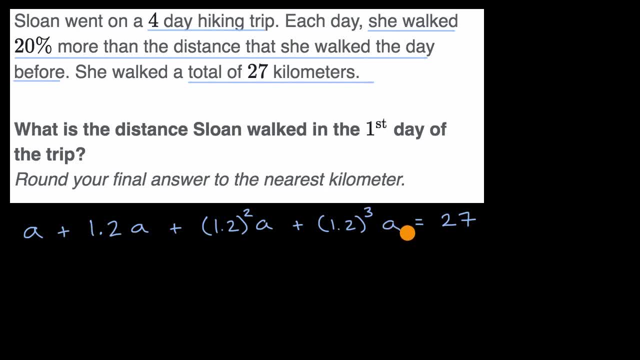 Now you could solve for a over here. You could factor out the a and you could say: a times one plus 1.2, plus 1.2 squared plus 1.2 to the third power is equal to 27.. And then you could say that a is equal to 1.2 squared. 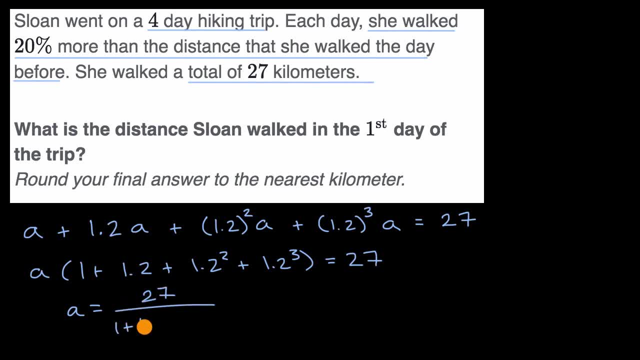 That's equal to 27 over one plus 1.2, plus 1.2 squared plus 1.2 to the third power, And we would need a calculator to evaluate this. But I'm going to do a different technique, a technique that would work even if you had 20 terms here. 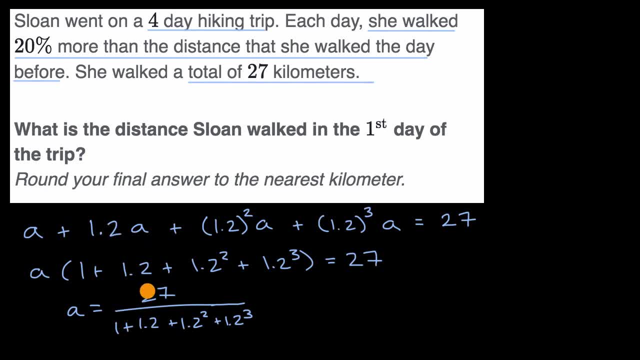 You, in theory, could also do this with 20 terms, but it gets a lot more complicated, or if you had 200 terms. So the other way to approach this is use the formula for a finite geometric series. What does it evaluate to? 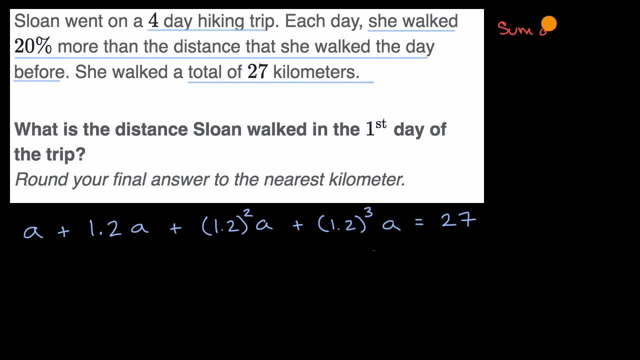 And, just as a reminder, the sum of first n terms. it's going to be the first term which we could call a minus. the first term times our common ratio. In this case, our common ratio is 1.2, because every successive term is 1.2 times the first. 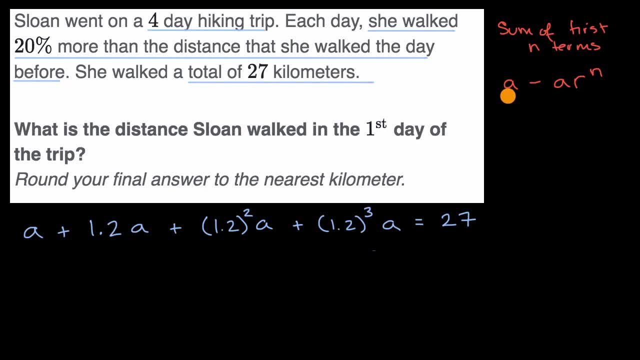 So our first term times our common ratio to the nth power. All of that over one, minus the common ratio. In other videos we explain where this comes from, We prove this, But here we can just apply it. We already know what our a is. 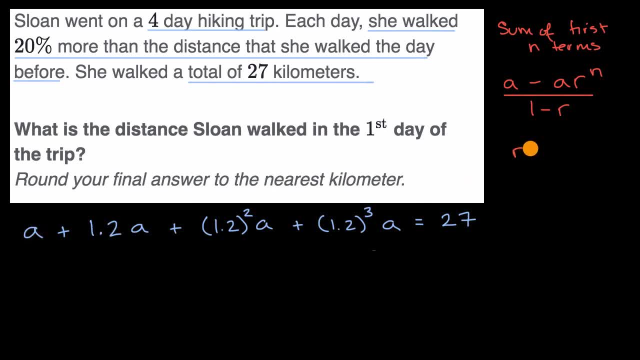 I use that as our variable. Our common ratio in this situation is going to be equal to 1.2.. And our n is going to be equal to four. Another way I like to think about it is: it's our first term which we see right over there. 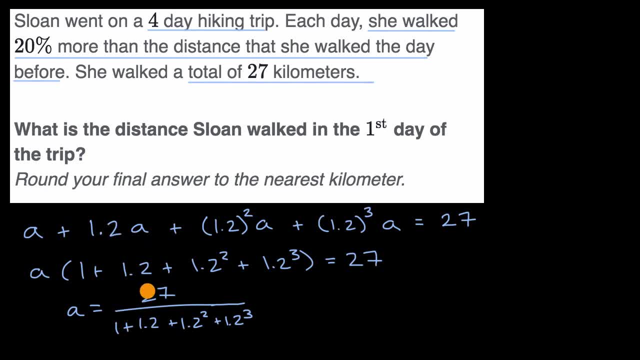 You, in theory, could also do this with 20 terms, but it gets a lot more complicated, or if you had 200 terms. So the other way to approach this is use the formula for a finite geometric series. What does it evaluate to? 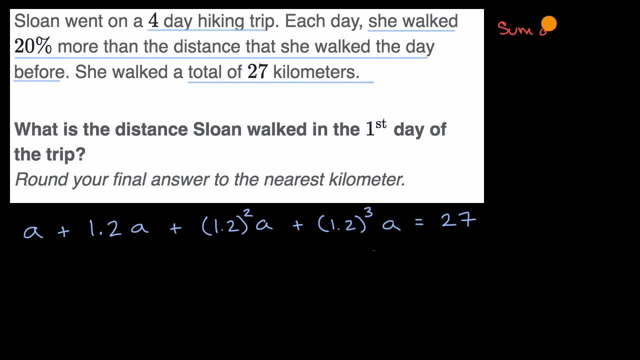 And, just as a reminder, the sum of first n terms. it's going to be the first term which we could call a minus. the first term times our common ratio. In this case, our common ratio is 1.2, because every successive term is 1.2 times the first. 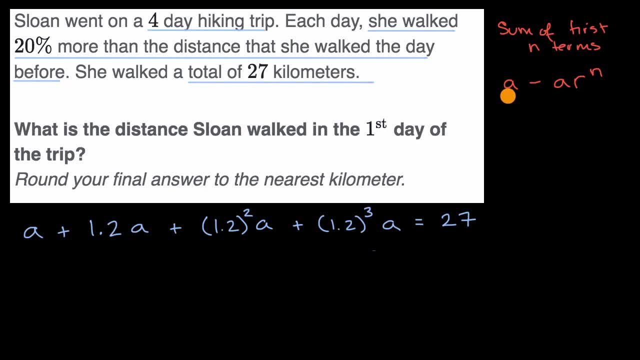 So our first term times our common ratio to the nth power. All of that over one, minus the common ratio. In other videos we explain where this comes from, We prove this, But here we can just apply it. We already know what our a is. 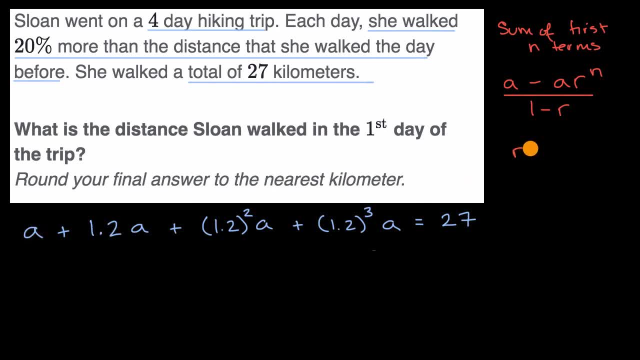 I use that as our variable. Our common ratio in this situation is going to be equal to 1.2.. And our n is going to be equal to four. Another way I like to think about it is: it's our first term which we see right over there. 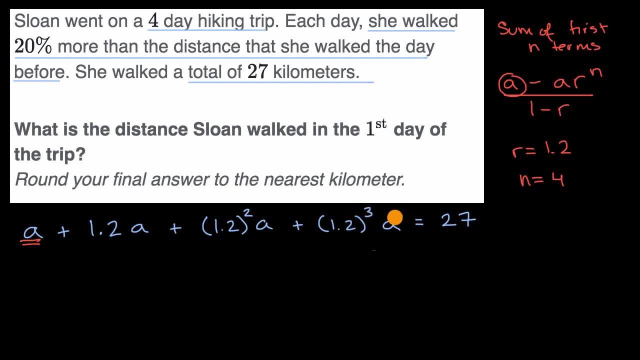 minus the term that we did not get. If we did not get to, if we were to have a fifth term, it would have been that fifth term that we're subtracting because we aren't getting to a fourth power here. The fifth term would have been to the fourth power. 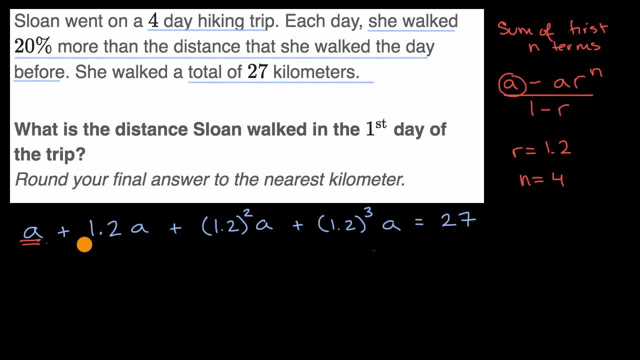 All of that over one minus the common ratio. And so this left-hand side of our equation we could rewrite as our first term minus our first term times our common ratio 1.2, to the fourth power. All of that over one minus the fourth power. 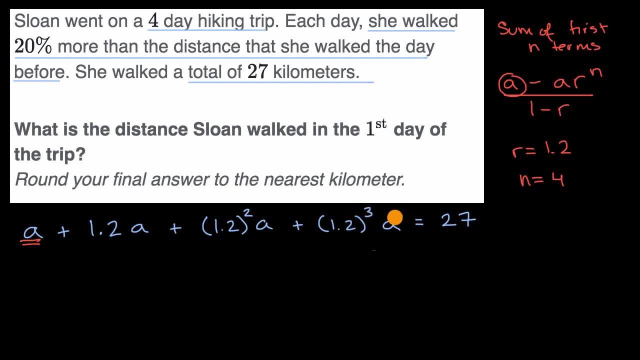 minus the term that we did not get. If we did not get to, if we were to have a fifth term, it would have been that fifth term that we're subtracting because we aren't getting to a fourth power here. The fifth term would have been to the fourth power. 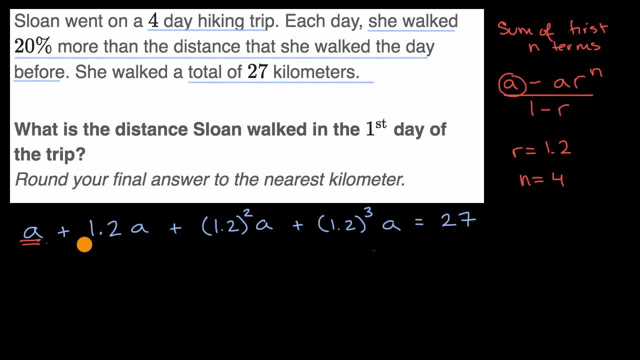 All of that over one minus the common ratio. And so this left-hand side of our equation we could rewrite as our first term minus our first term times our common ratio 1.2, to the fourth power. All of that over one minus the fourth power. 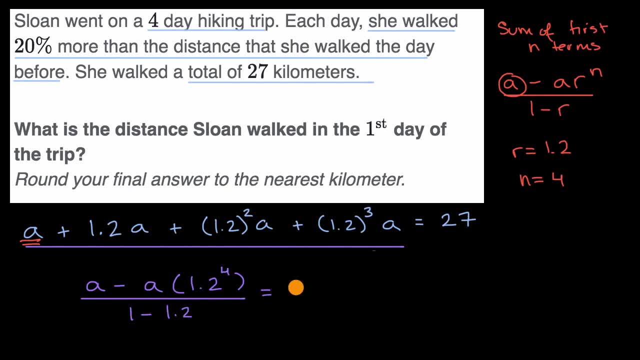 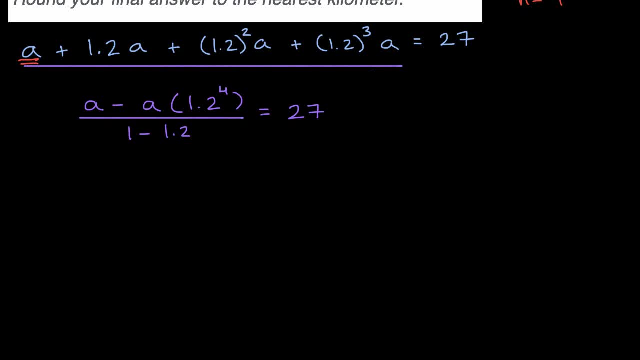 All of that over one minus the fourth power, All of that over one minus our common ratio, And then that could be equal to 27.. Let me scroll down a little bit so we have some more space to then solve this. And so let's see, I can simplify this a little bit. 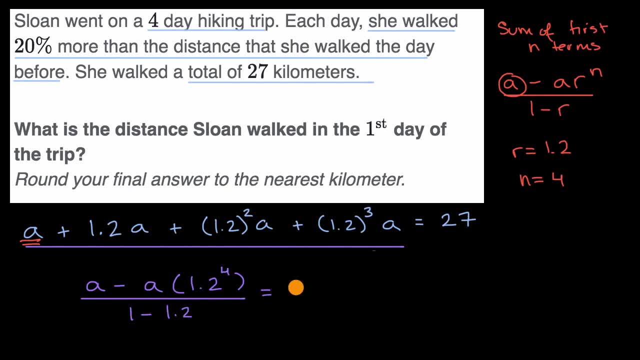 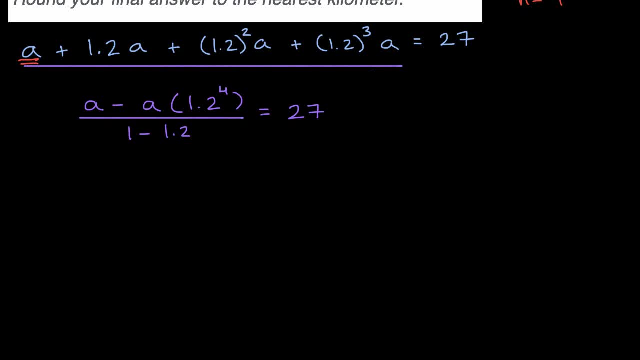 All of that over one minus the fourth power, All of that over one minus our common ratio, And then that could be equal to 27.. Let me scroll down a little bit so we have some more space to then solve this. And so let's see, I can simplify this a little bit. 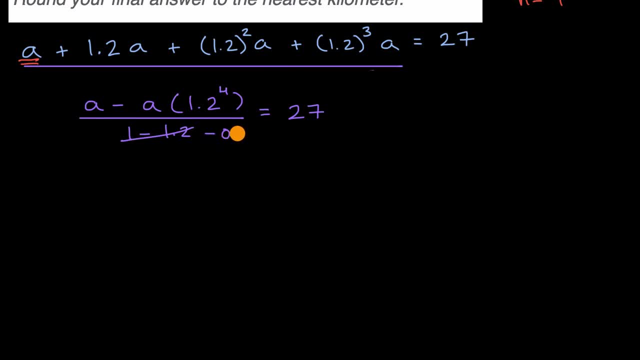 We could. this is going to be equal to negative 0.2., Our numerator. we can factor out an, a, And so this is going to be equal to a times one minus 1.2, to the fourth power, And let's see, we can multiply. 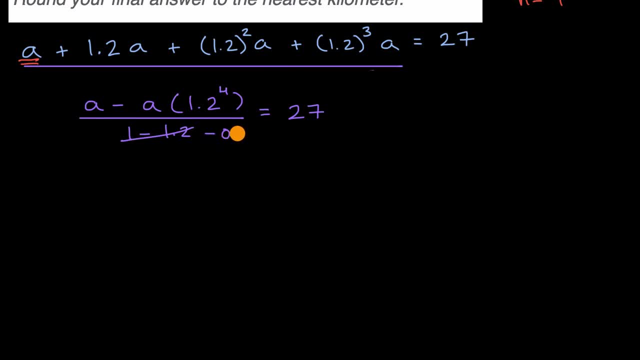 We could. this is going to be equal to negative 0.2., Our numerator. we can factor out an, a, And so this is going to be equal to a times one minus 1.2, to the fourth power, And let's see, we can multiply. 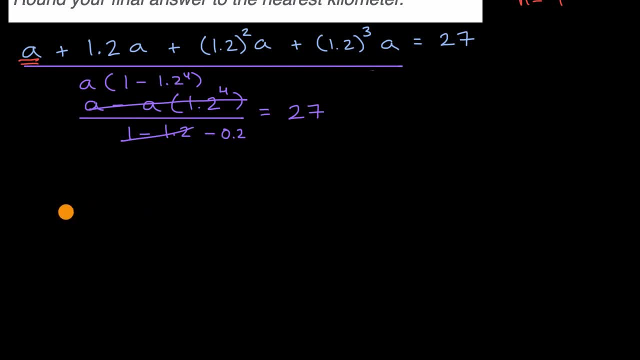 both the numerator and the denominator by a negative one, And so this would get us to a times a times, and I'll put the a out of the fraction a times. so I'll just swap the order here and get rid of this negative. 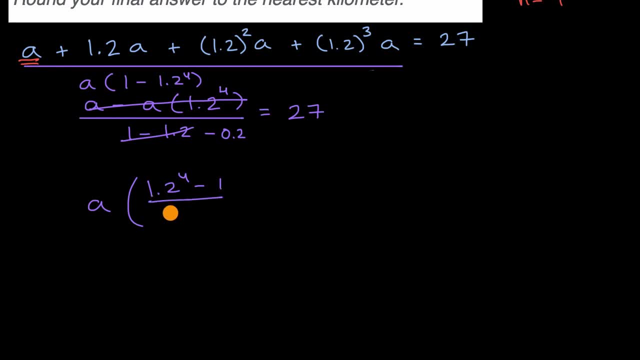 1.2 to the fourth. power minus one over 0.2 is equal to 27.. Again, all I did is I took the a out of the fraction, so it's out here, and I multiplied the numerator and the denominator by a negative. 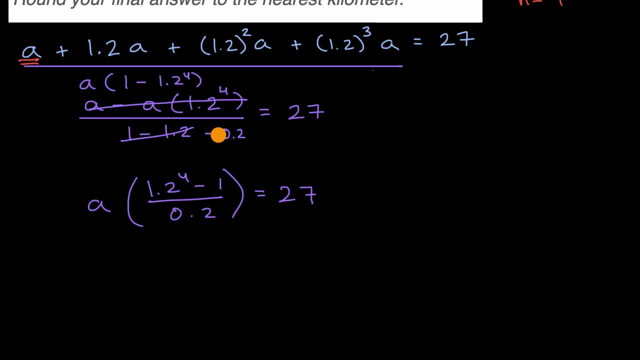 The numerator multiplied by a negative would swap these two, And then multiplying negative 0.2 times a negative is just positive 0.2.. And so now I can just multiply both sides times the reciprocal of this. So I'll do it here. 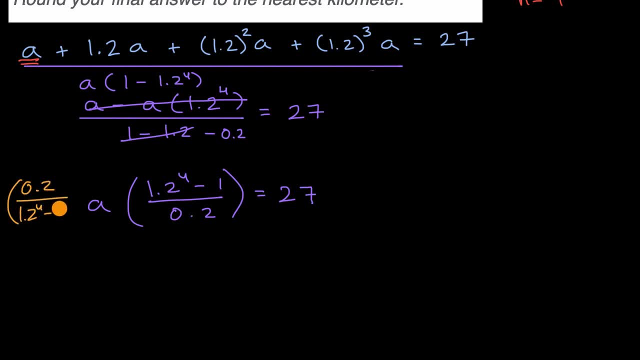 So 0.2 over 1.2 to the fourth minus one. And then here, 0.2 over 1.2 to the fourth minus one. That cancels with that. that cancels with that. That's exactly why I did that. 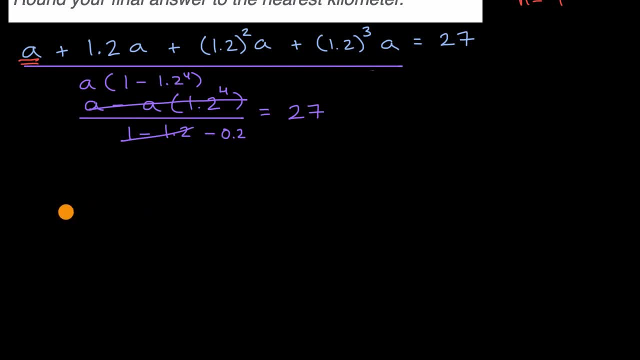 both the numerator and the denominator by a negative one, And so this would get us to a times a times, and I'll put the a out of the fraction a times. so I'll just swap the order here and get rid of this negative. 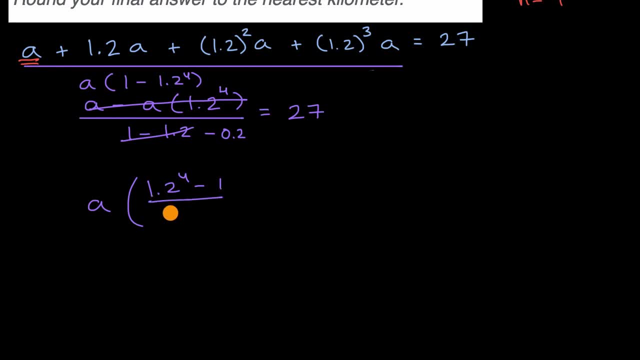 1.2 to the fourth. power minus one over 0.2 is equal to 27.. Again, all I did is I took the a out of the fraction, so it's out here, and I multiplied the numerator and the denominator by a negative. 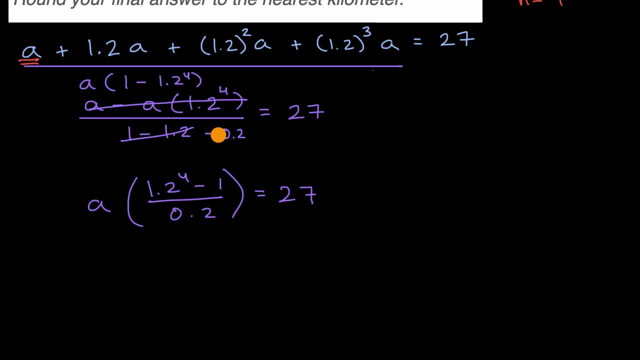 The numerator multiplied by a negative would swap these two, And then multiplying negative 0.2 times a negative is just positive 0.2.. And so now I can just multiply both sides times the reciprocal of this. So I'll do it here. 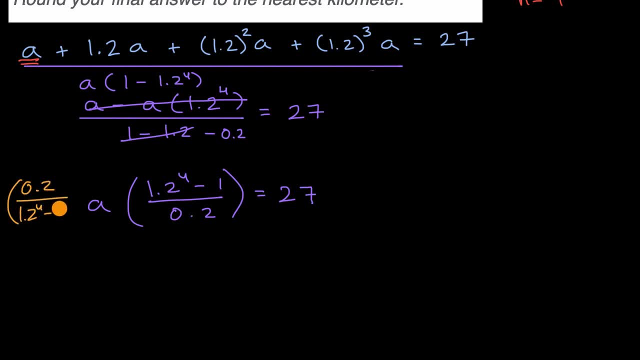 So 0.2 over 1.2 to the fourth minus one. And then here, 0.2 over 1.2 to the fourth minus one. That cancels with that. that cancels with that. That's exactly why I did that. 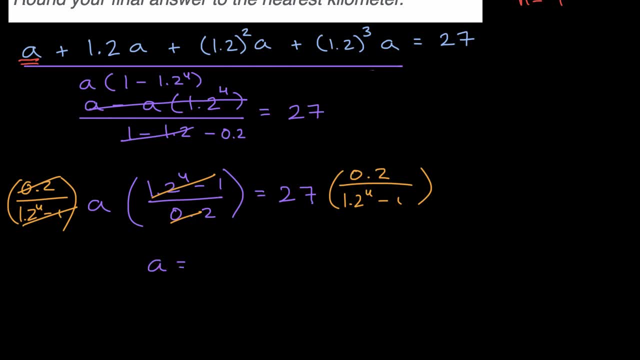 And we're left with a is equal to, it is equal to- I'll just write it in yellow: 27 times 0.2, all of that over 1.2 to the fourth minus one, And this expression should give us the exact same value. 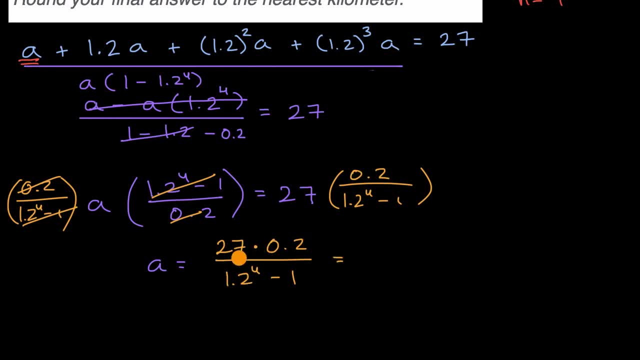 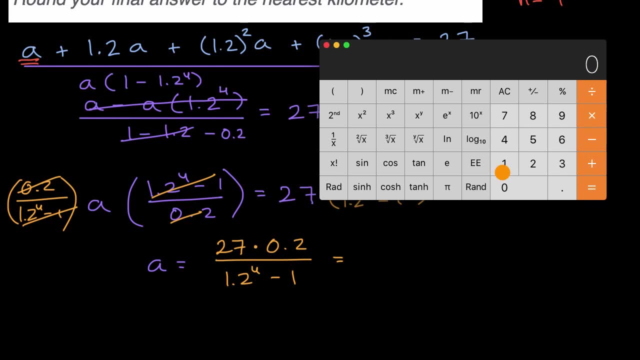 as that expression we just saw. But this is useful. even if we had 100 terms, we could use this, And so I'll get the calculator out. This will give us, so I will actually I'll evaluate this denominator first, So I'll have 1.2 to the fourth power. 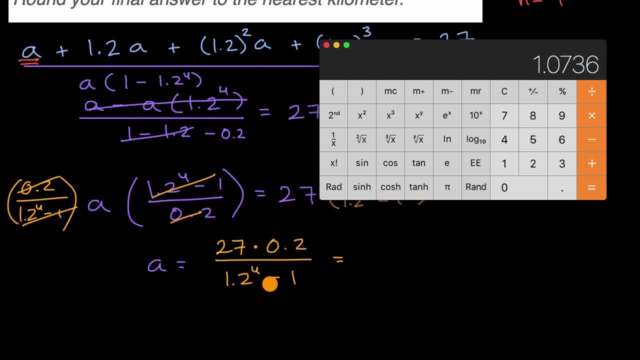 which is equal to minus one, is equal to. now it's in the denominator, so I could just take the reciprocal of it And then multiply that times 27 times 0.2 is equal to 5.029.. Now they want us to round our answer. 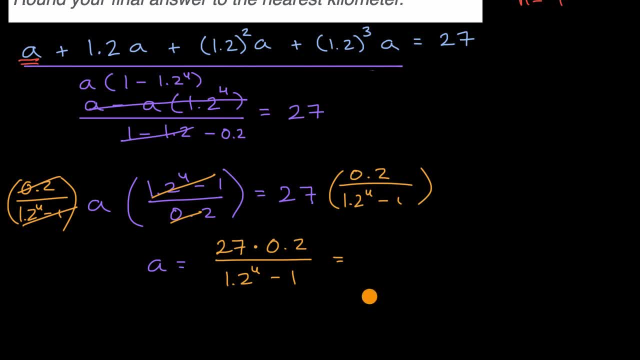 to the nearest kilometer. so this is going to be approximately equal to approximately equal to five kilometers. That's how much approximately that she would have traveled on the first day of her hiking trip. 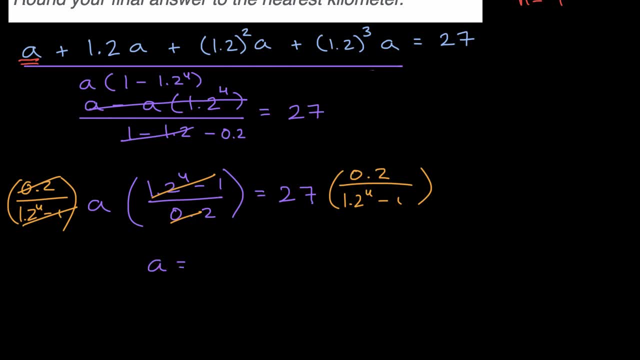 And we're left with a is equal to, it is equal to- I'll just write it in yellow: 27 times 0.2, all of that over 1.2 to the fourth minus one, And this expression should give us the exact same value. 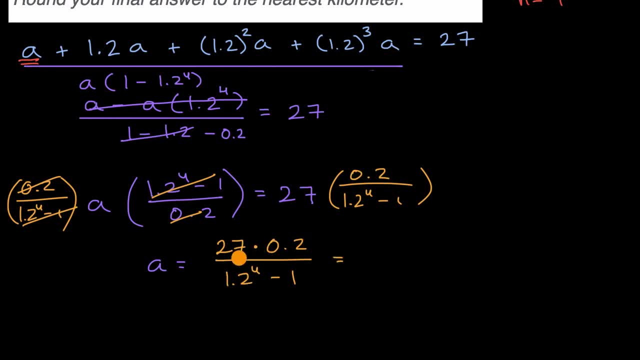 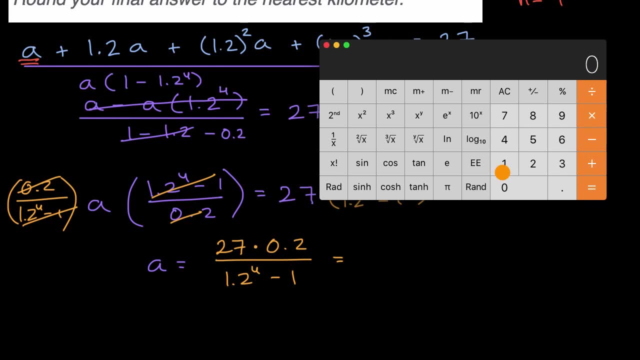 as that expression we just saw. But this is useful. even if we had 100 terms, we could use this, And so I'll get the calculator out. This will give us, so I will actually I'll evaluate this denominator first, So I'll have 1.2 to the fourth power. 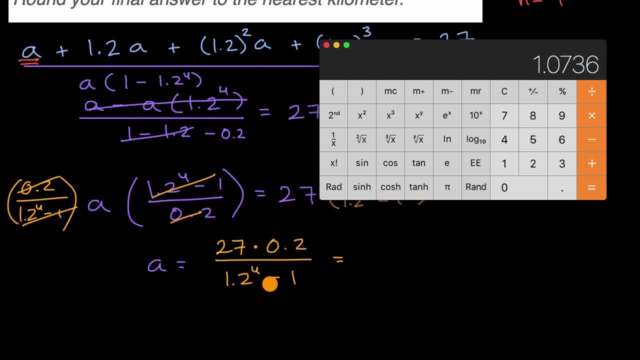 which is equal to minus one, is equal to. now it's in the denominator, so I could just take the reciprocal of it And then multiply that times 27 times 0.2 is equal to 5.029.. Now they want us to round our answer.